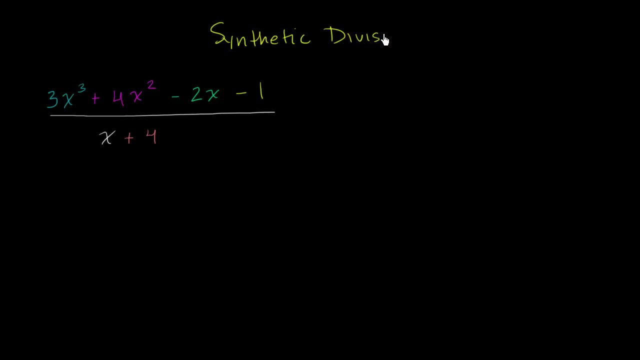 And synthetic division is going to seem like a little bit of voodoo in the context of this video. In the next few videos we're going to think about why it actually makes sense, why you actually get the same result as traditional algebraic long division. 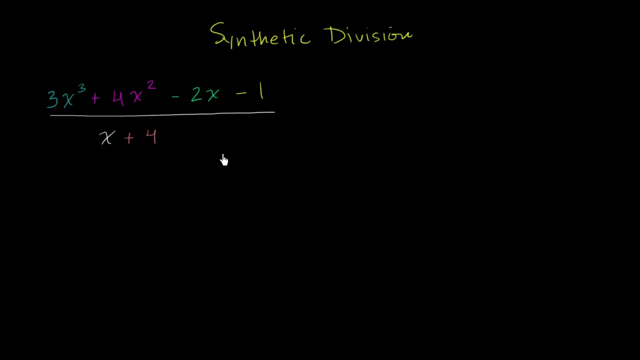 My personal tastes are not to like synthetic division because it is very, very, very algorithmic. I prefer to do traditional algebraic long division. But I think you'll see that this has some advantages: It can be faster and it also uses. 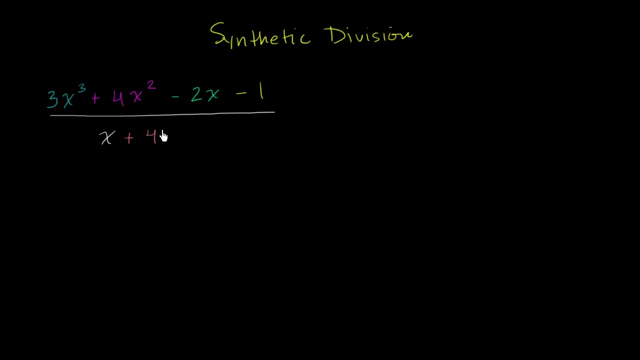 a lot less space on your paper. So let's actually perform this synthetic division, Let's actually simplify this expression. Before we start, there's two important things to keep in mind. We're doing kind of the most basic form of synthetic division. 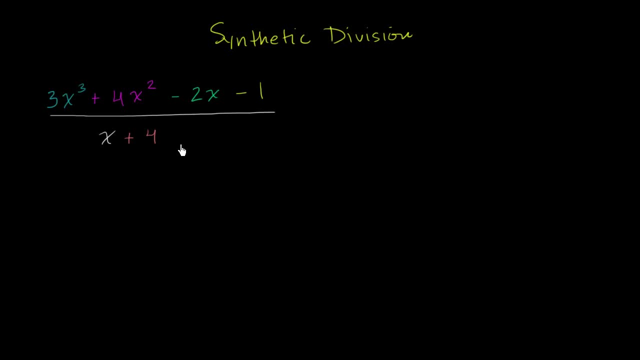 And to do this most basic algorithm, this most basic algorithm, we're going to need to do a few things. We're going to need to do a few things. This is a basic process. You have to look for two things in this bottom expression. 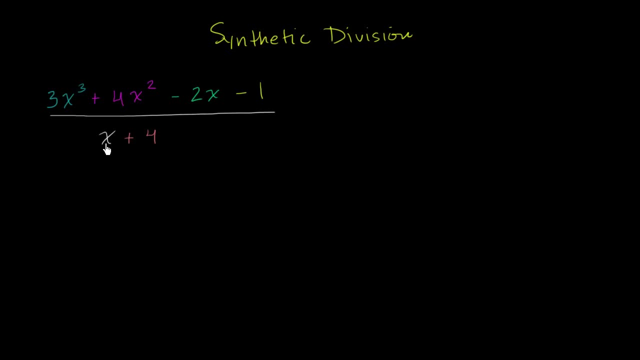 The first is that it has to be a polynomial of degree 1.. So you have just an x here. You don't have an x squared, an x to the third, an x to the fourth or anything like that. The other thing is that the coefficient here is a 1.. 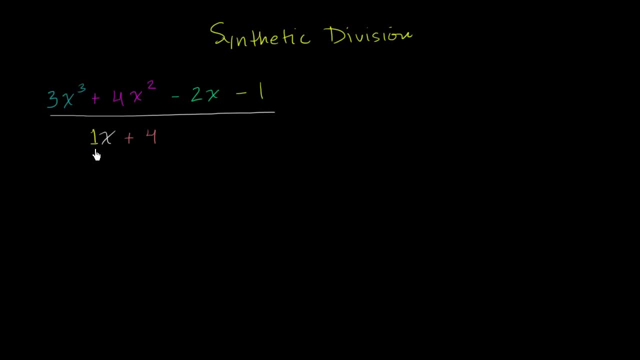 There are ways to do it if the coefficient was different, but then our synthetic division will have to add a little bit of bells and whistles to it. So in general, what I'm going to show you now will work. You have something of the form x plus or minus, something else. 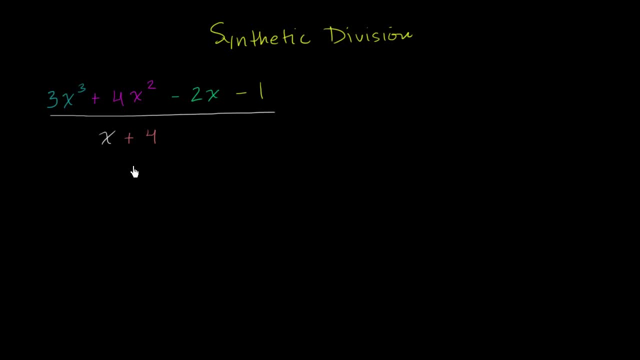 So, with that said, let's actually perform the synthetic division. So the first thing I'm going to do is write all the coefficients for this polynomial that's in the numerator. So let's write all of them, So we have a 3.. 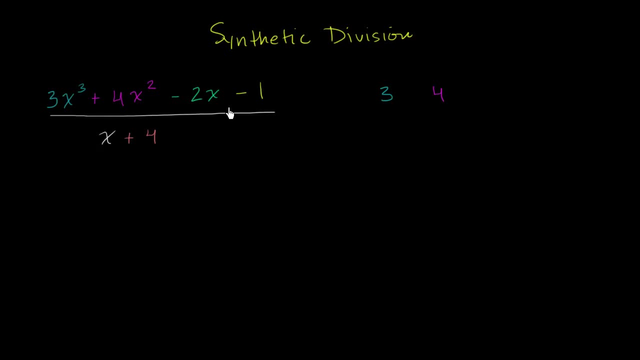 We have a 4.. It's a positive 4.. We have a negative 2 and a negative 1.. And you'll see different people draw different types of signs here, depending on how they're doing synthetic division, but this is the most traditional. 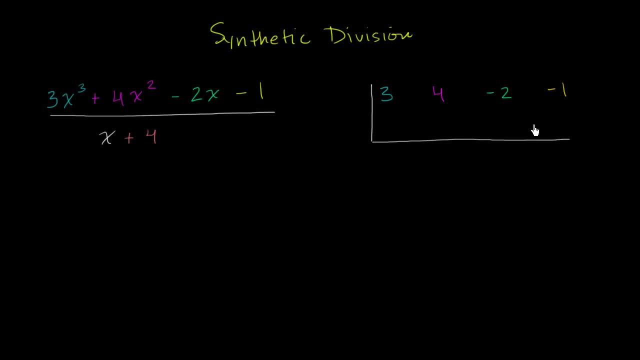 And you want to leave some space right here for another row of numbers. So that's why I've gone all the way down here. And then we look at the denominator And in particular, we're going to look whatever x, plus or minus is right over here. 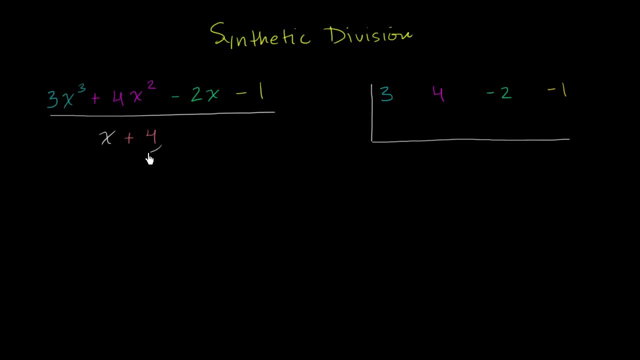 So we'll look at right over here we have a positive 4.. Instead of writing a positive 4, we write the negative of that. So we write the negative of x plus or minus 4.. So we write the negative of x plus or minus 4.. 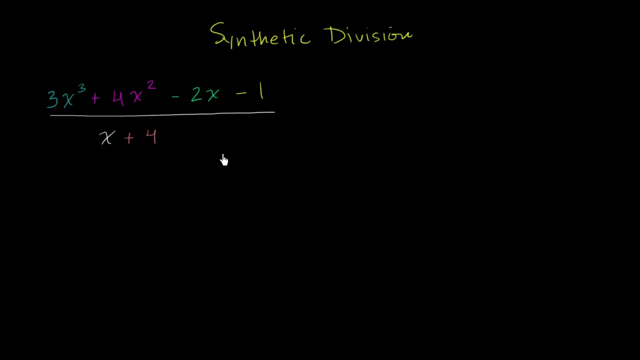 My personal tastes are not to like synthetic division because it is very, very, very algorithmic. I prefer to do traditional algebraic long division. But I think you'll see that this has some advantages: It can be faster and it also uses. 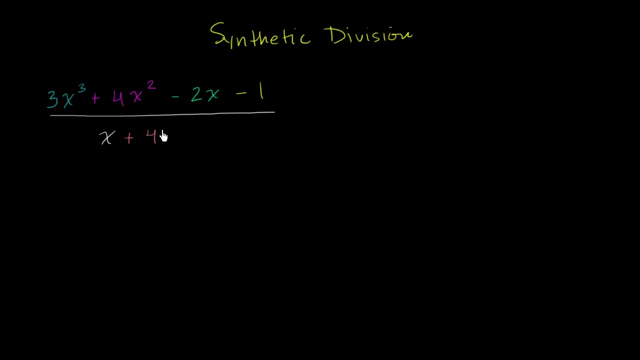 a lot less space on your paper. So let's actually perform this synthetic division, Let's actually simplify this expression. Before we start, there's two important things to keep in mind. We're doing kind of the most basic form of synthetic division. 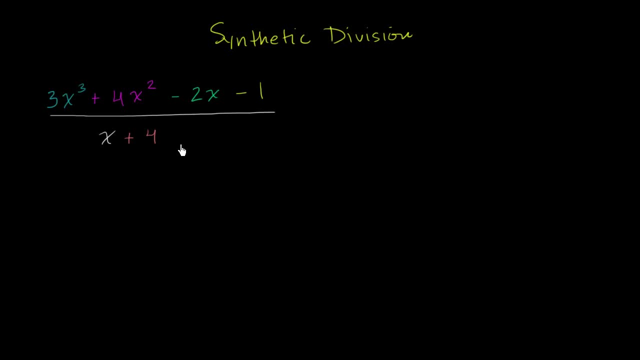 And to do this most basic algorithm, this most basic algorithm, we're going to need to do a few things. We're going to need to do a few things. This is a basic process. You have to look for two things in this bottom expression. 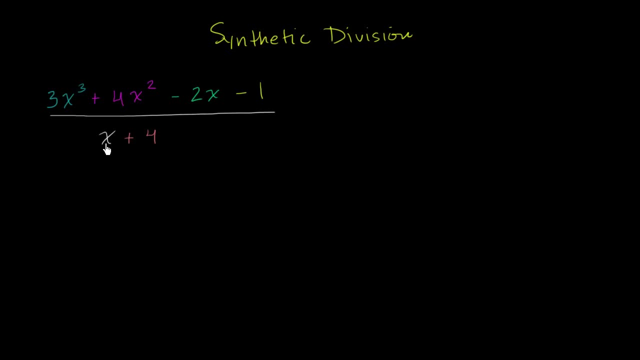 The first is that it has to be a polynomial of degree 1.. So you have just an x here. You don't have an x squared, an x to the third, an x to the fourth or anything like that. The other thing is that the coefficient here is a 1.. 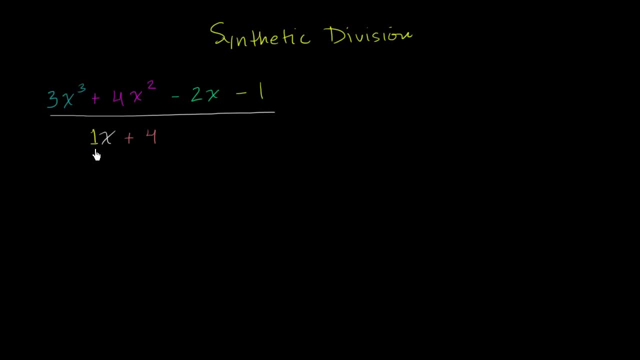 There are ways to do it if the coefficient was different, but then our synthetic division will have to add a little bit of bells and whistles to it. So in general, what I'm going to show you now will work. You have something of the form x plus or minus, something else. 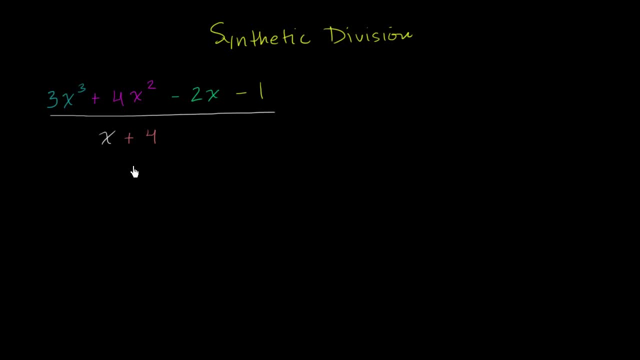 So, with that said, let's actually perform the synthetic division. So the first thing I'm going to do is write all the coefficients for this polynomial that's in the numerator. So let's write all of them, So we have a 3.. 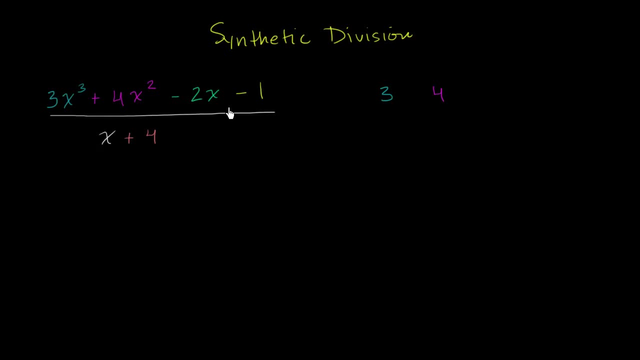 We have a 4.. It's a positive 4.. We have a negative 2 and a negative 1.. And you'll see different people draw different types of signs here, depending on how they're doing synthetic division, but this is the most traditional. 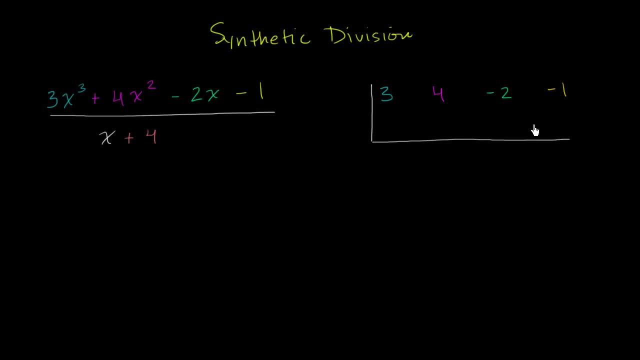 And you want to leave some space right here for another row of numbers. So that's why I've gone all the way down here. And then we look at the denominator And in particular, we're going to look whatever x, plus or minus is right over here. 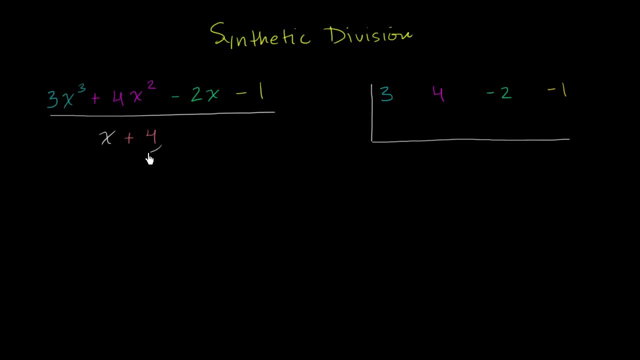 So we'll look at right over here we have a positive 4.. Instead of writing a positive 4, we write the negative of that. So we write the negative of x plus or minus 4.. So we write the negative of x plus or minus 4.. 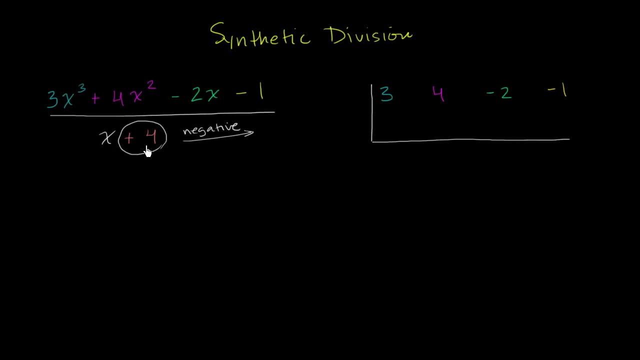 So we write the negative of x plus or minus 4.. We write the negative of that which would be negative 4.. We write negative 4.. And now we are all set up and we are ready to perform our synthetic division. 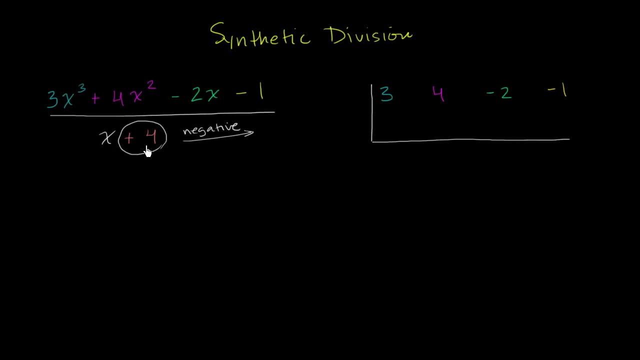 So we write the negative of x plus or minus 4.. We write the negative of that which would be negative 4.. We write negative 4.. And now we are all set up and we are ready to perform our synthetic division. 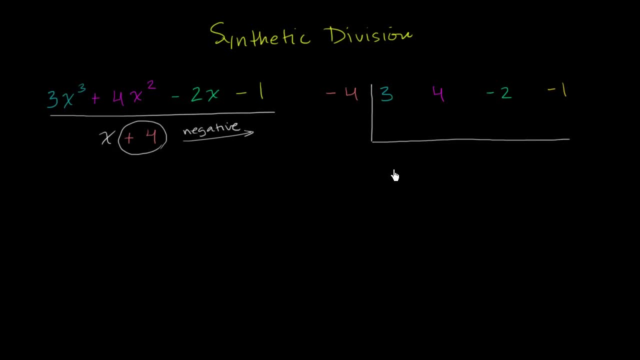 And it's going to seem like voodoo. In future videos we'll explain why this works. So first this first coefficient. we literally just bring it straight down, And so you put the 3 there. Then you multiply what you have here, times the negative 4.. 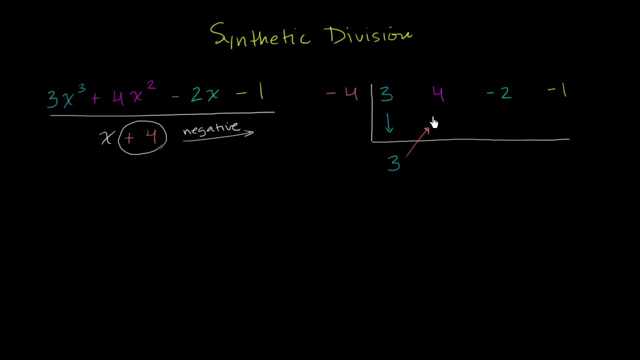 So you multiply it times the negative 4.. 3 times negative: 4 is negative 12. Then you add the 4 to the negative 12.. 4 plus negative: 12 is negative 8.. Then you multiply negative 8 times the negative 4.. 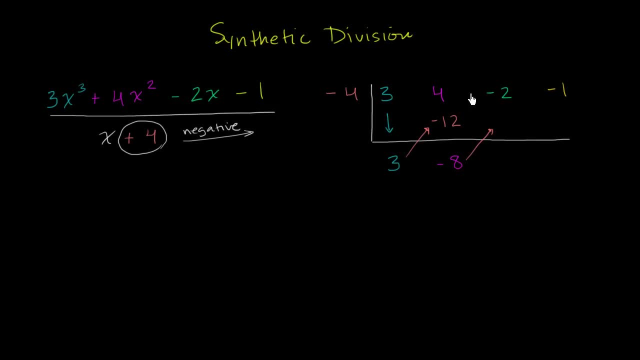 I think you see the pattern: Negative 8 times negative 4 is positive 32.. Now we add negative 2 plus positive 32. That gives us positive 30. Then you multiply the positive 32.. Positive 30 times the negative 4.. 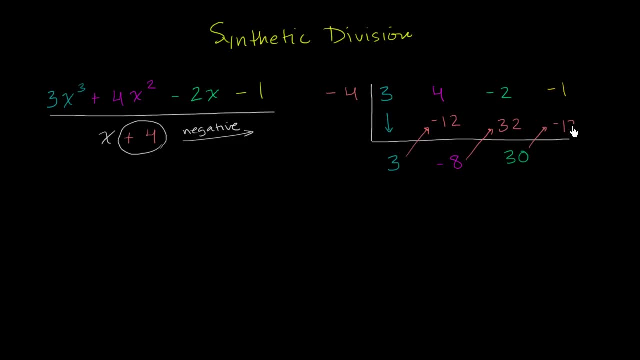 And that gives you negative 120. And then you add the negative 1 plus the negative 120. And you end up with a negative 121.. And now the last thing you do is you say: well, I have one term here. 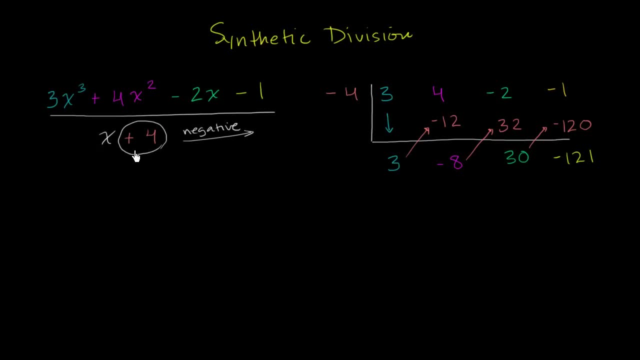 And in this plain vanilla, simple version of synthetic division we're only dealing actually when you have x plus or minus something. So you're only going to have one term there. So you separate out 1.. You separate out 1 term from the right, just like that. 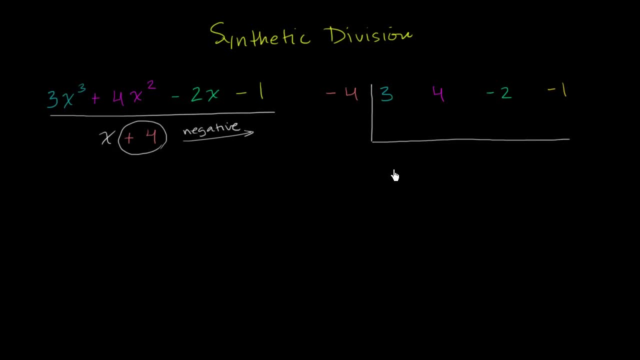 And it's going to seem like voodoo. In future videos we'll explain why this works. So first this first coefficient. we literally just bring it straight down, And so you put the 3 there. Then you multiply what you have here, times the negative 4.. 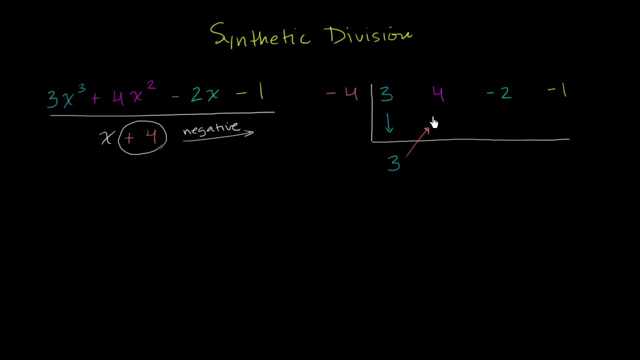 So you multiply it times the negative 4.. 3 times negative: 4 is negative 12. Then you add the 4 to the negative 12.. 4 plus negative: 12 is negative 8.. Then you multiply negative 8 times the negative 4.. 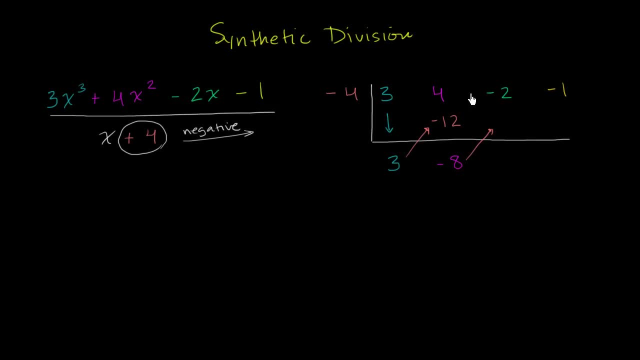 I think you see the pattern: Negative 8 times negative 4 is positive 32.. Now we add negative 2 plus positive 32. That gives us positive 30. Then you multiply the positive 32.. Positive 30 times the negative 4.. 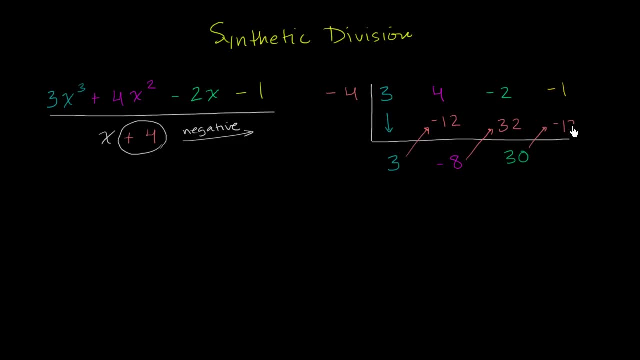 And that gives you negative 120. And then you add the negative 1 plus the negative 120. And you end up with a negative 121.. And now the last thing you do is you say: well, I have one term here. 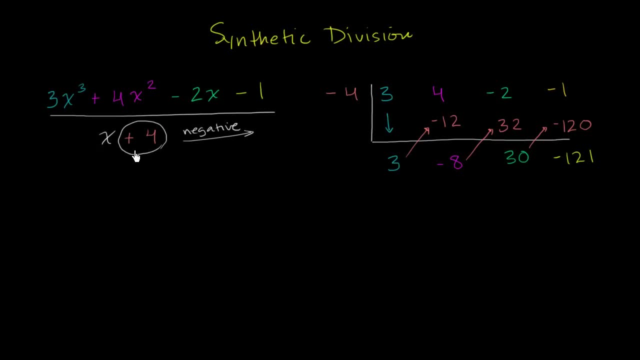 And in this plain vanilla, simple version of synthetic division we're only dealing actually when you have x plus or minus something. So you're only going to have one term there. So you separate out 1.. You separate out 1 term from the right, just like that. 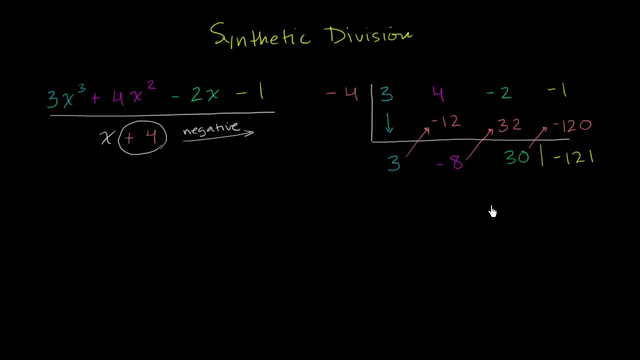 And we essentially have our answer, even though it seems like voodoo. So, to simplify this, you get and you can have a drum roll right over here. This is going to be the constant term. You could think of it a degree 0 term. 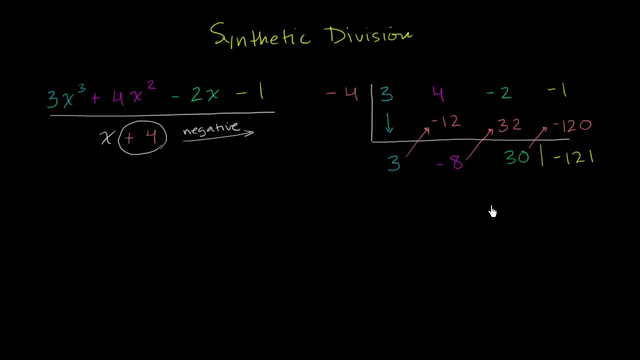 And we essentially have our answer, even though it seems like voodoo. So, to simplify this, you get and you can have a drum roll right over here. This is going to be the constant term. You could think of it a degree 0 term. 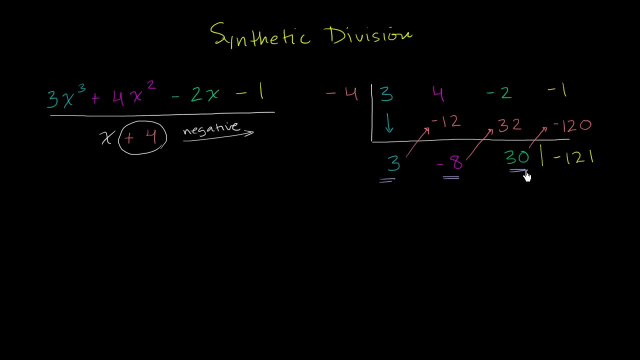 This is going to be an x term And this is going to be an x squared term. You can kind of just build up from here saying this: first one's going to be constant, Then this is going to be an x term, then an x squared. 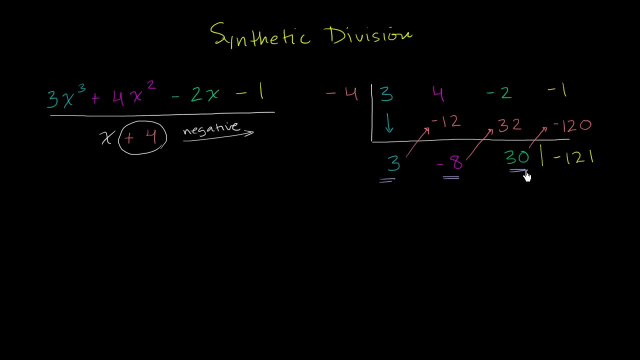 This is going to be an x term And this is going to be an x squared term. You can kind of just build up from here saying this: first one's going to be constant, Then this is going to be an x term, then an x squared. 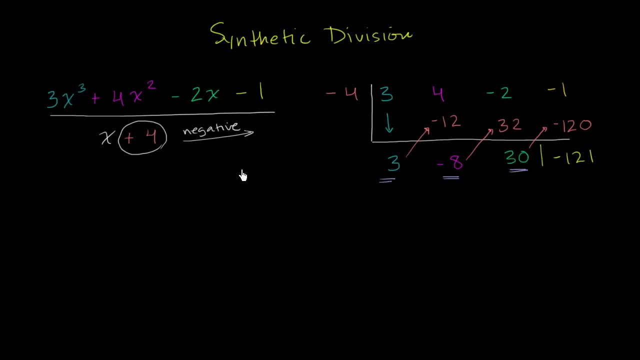 If we had more, you'd have an x to the third, an x to the fourth, so on and so forth. So this is going to be equal to 3x squared minus 8x plus 30.. And this right over here you can view as the remainder.